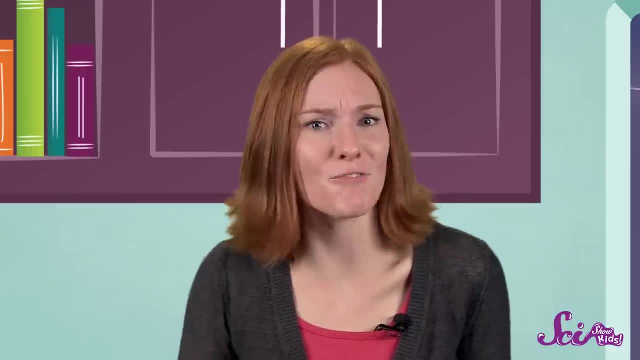 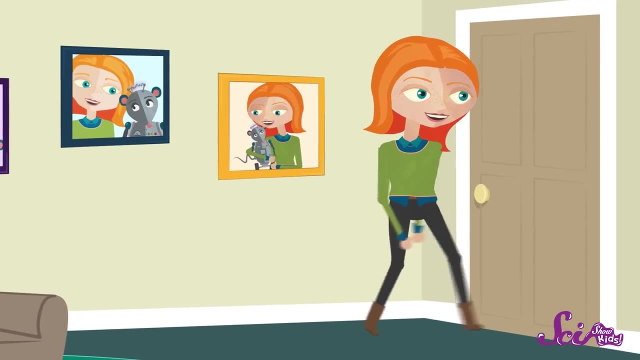 and the big booms that follow. And you may not know it, but the science of what causes lightning can happen right in your own home. Have you ever walked across a fuzzy carpet and then, when you reach for a doorknob, gotten? 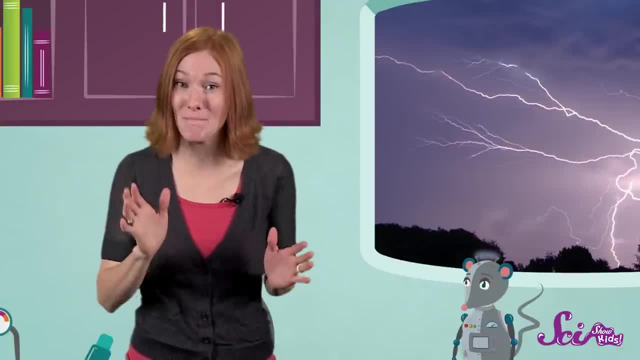 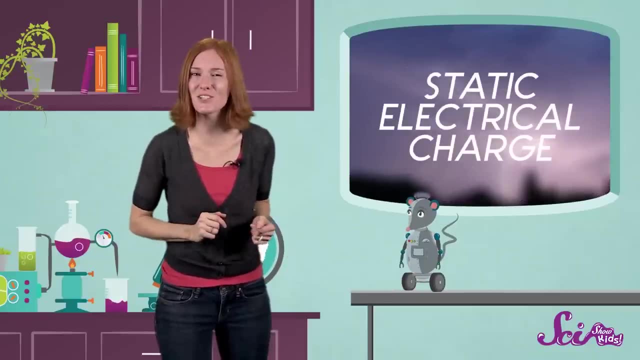 a little shock. If so, then you've been part of making a mini lightning bolt. That shock that you felt was caused by the buildup of what's known as a static electrical charge. A static electrical charge is just a little bit of electricity that stays in. 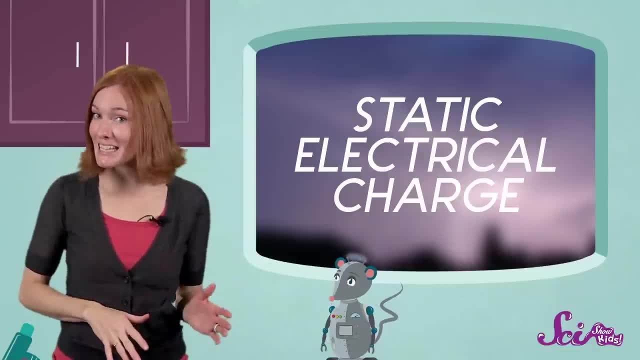 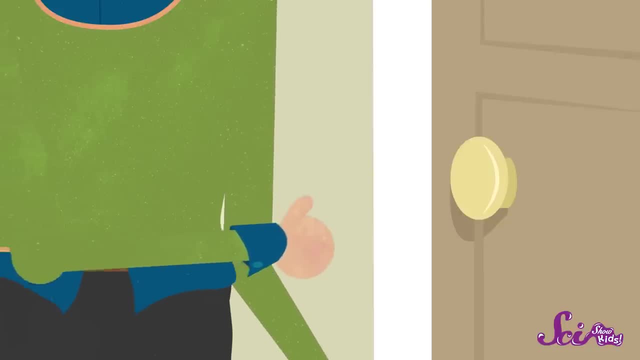 one place for a little, while Static electricity can build up any time. two things rub together: When you walk across the carpet, your body picks up tiny bits of charge. Then, when you reach for that doorknob, these charges jump into the metal doorknob and zap. 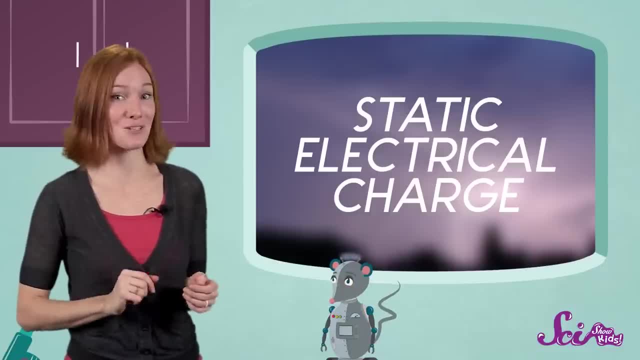 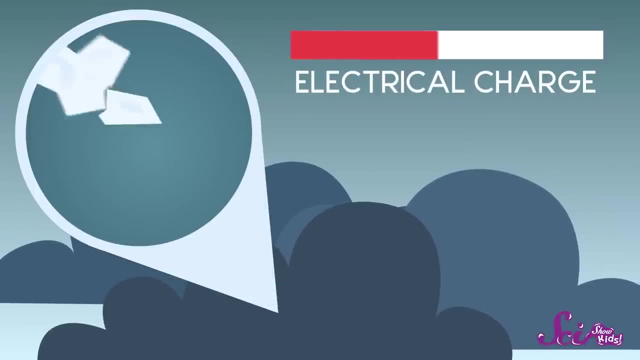 Lightning is caused by the same thing, only on a much bigger scale. The kinds of clouds we see in thunderstorms have tiny bits of ice in them And these little bits of ice bump into each other. They cause an electrical charge to build up inside the 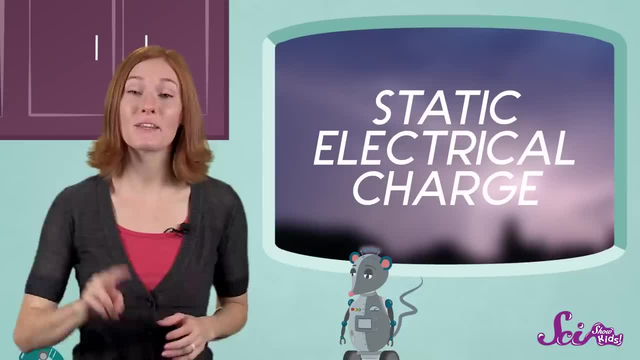 cloud And as this charge keeps building up, it gets stronger. But there are two kinds of electrical charge. We call them positive and negative. Charges that are different from one another will interact with each other And they're different from one another. 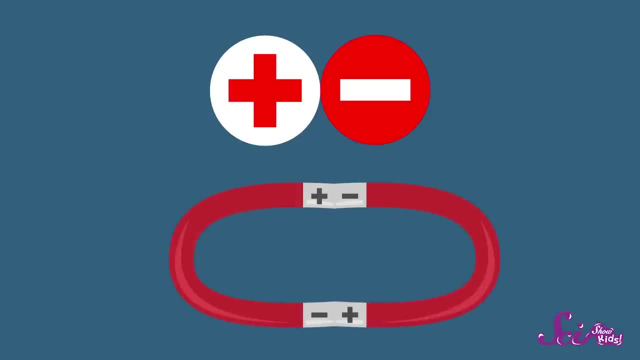 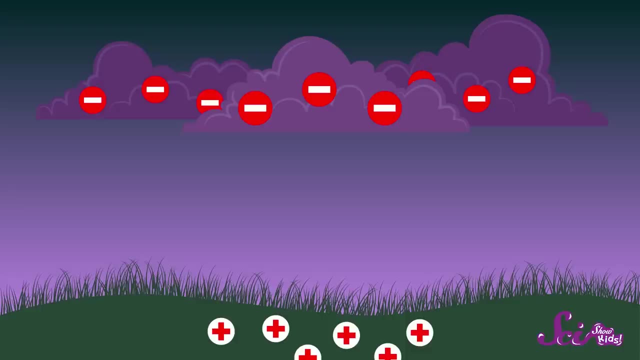 attract or pull toward one another, a lot like magnets, But in our case the charge in the cloud is negative. The negative charge in the cloud makes some spots on the ground get a positive charge And when the charges in the cloud and the charges on the ground are just right, a bolt. 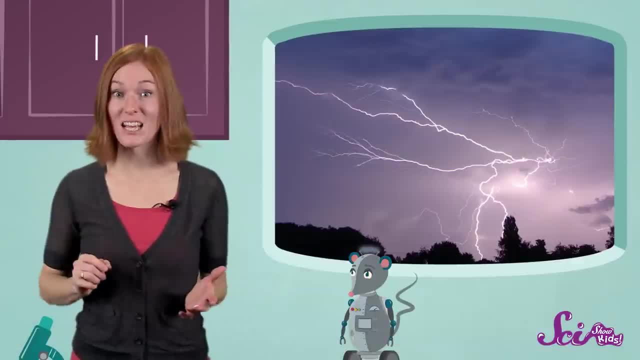 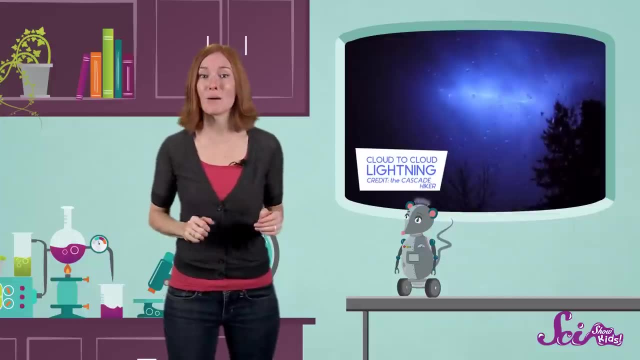 of lightning jumps between the cloud and the Earth, And meteorologists have discovered that there are different kinds of lightning too. Some lightning goes from one part of a cloud to another, some jumps from cloud to cloud, and some goes between the sky and the ground. 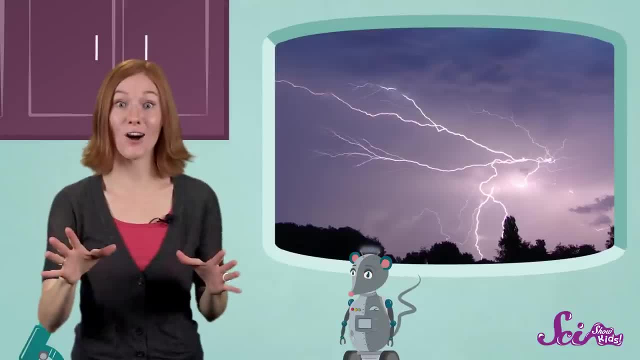 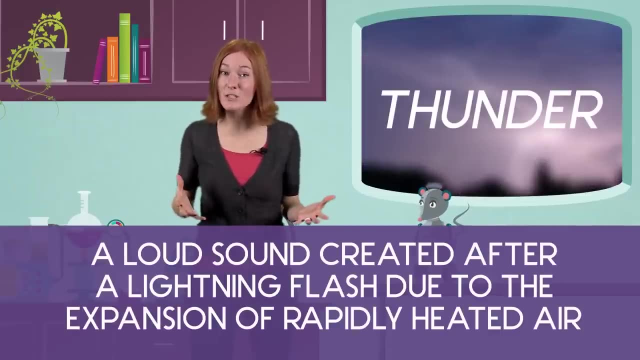 But it's all caused by a moving electrical charge, And all lightning is hot, Really hot, And that heat is what causes thunder. Thunder starts with the fact that air is made of tiny particles. When these little particles get heated up, they start to move around more quickly. So when the hot lightning bolt suddenly moves through the air, its heat makes the air particles around it all excited. All those particles of suddenly hot air start to move around quickly. They push hard against the cooler air around them. That air then flies away really fast from where the lightning is. 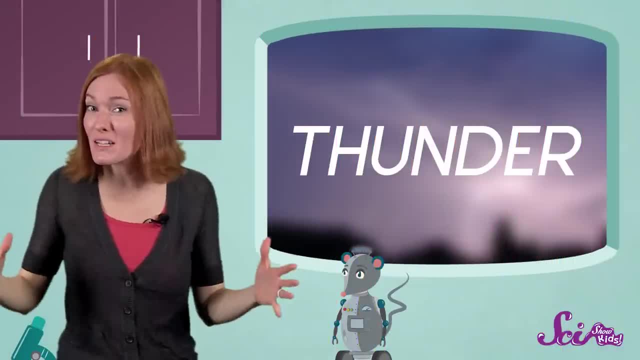 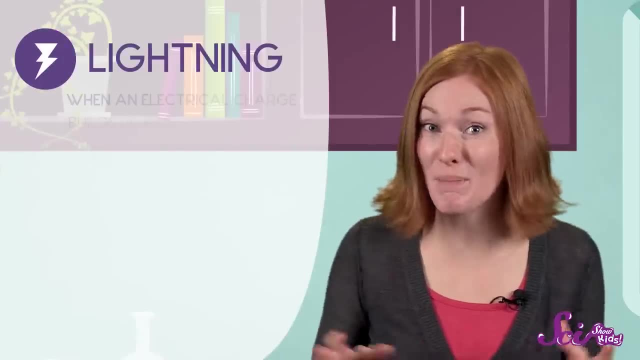 That's what lightning was with a lot of energy. Our ears hear this movement of the air particles as a loud bang or crackle. That's thunder. So now you know, Lightning happens when an electrical charge builds up inside of a cloud and moves to an 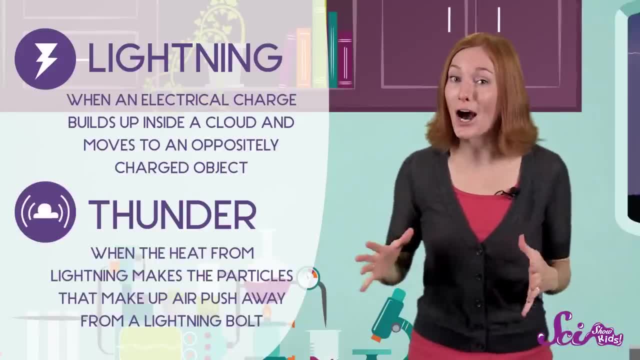 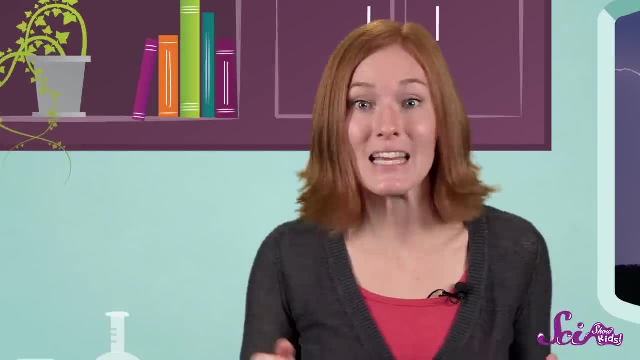 opposite charge And thunder happens when the heat from lightning causes the particles that make up air to push away from the lightning bolt. And remember, when you're not sure about something, ask questions. It just might make you feel better. Thanks for asking, Eleanor.